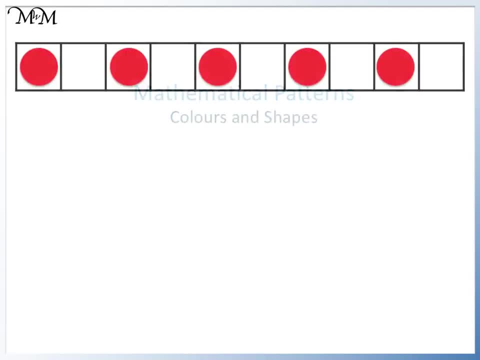 Hi and welcome to our lesson on mathematical shape patterns. Here is a set of red counters. After each red counter we will put a blue counter. We have a pattern which goes from red to blue. The pattern repeats with a red, then a blue, following each pair of red and blue. 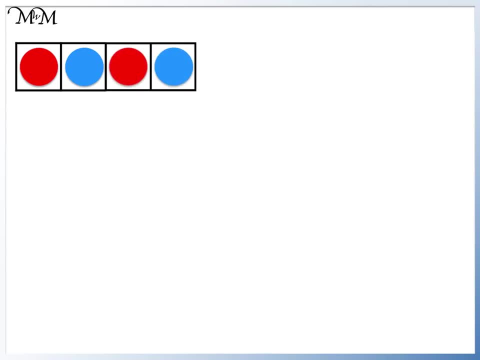 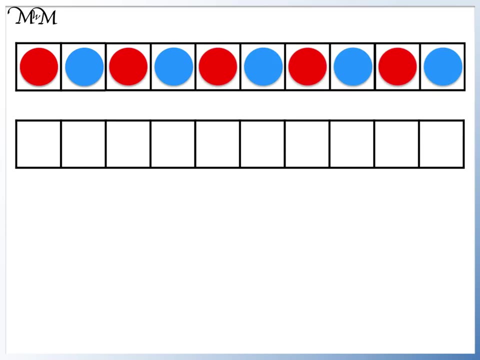 We can continue the pattern with blocks of red and blue. Here is a different pattern This time. we will start with a blue, We will follow with a red. We will make a pattern of blue and red. This pattern is formed by repeating blue, then red. 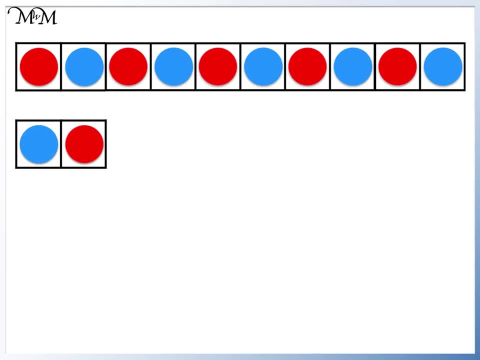 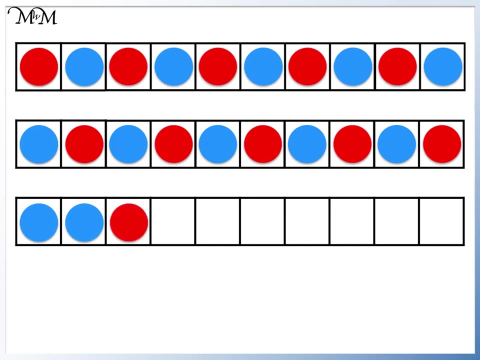 Instead of adding one colour at a time, we can add the blue followed by the red together. Here is a new pattern. We have blue, blue, red, red, Followed by blue, blue, red, red, Then another blue blue. 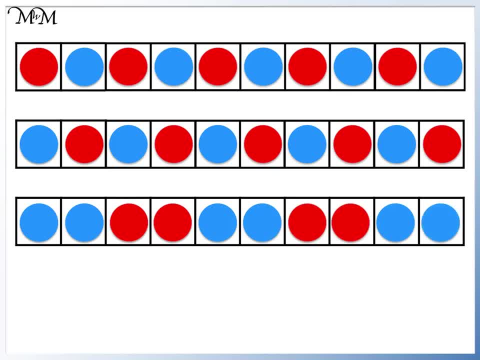 To see the pattern we look for which colours repeat. We have two blues and then two reds. This pattern repeats to create the sequence: We have blue blue, then red red, Next is blue blue. This pattern goes blue, blue, red, blue, blue, red, blue, blue red, followed by blue. 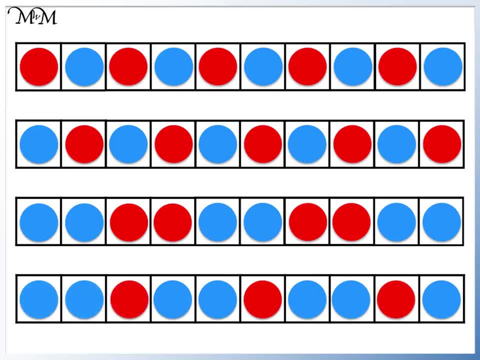 The repeating pattern is blue blue red. We can make the sequence from blue blue red, which repeats. after each red, We can add a blue blue red. After this red, we add a blue blue red. 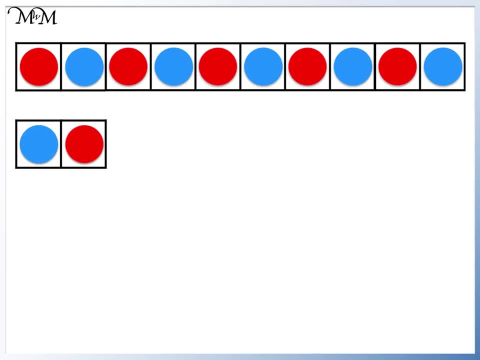 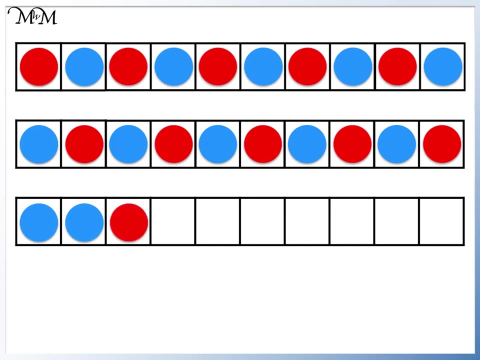 Instead of adding one colour at a time, we can add the blue followed by the red together. Here is a new pattern. We have blue, blue, red, red, Followed by blue, blue, red, red, Then another blue blue. 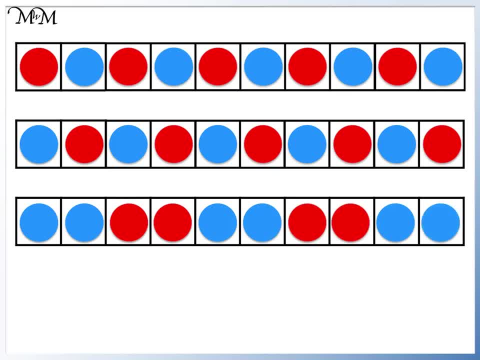 To see the pattern we look for which colours repeat. We have two blues and then two reds. This pattern repeats to create the sequence: We have blue blue, then red red, Next is blue blue. This pattern goes blue, blue, red, blue, blue, red, blue, blue red, followed by blue. 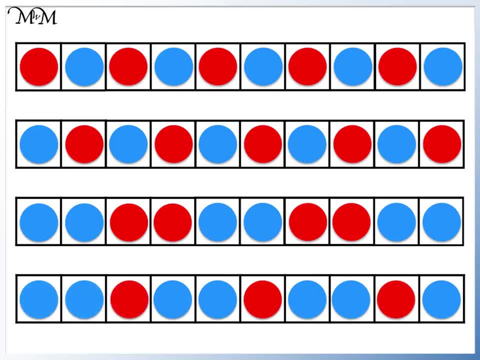 The repeating pattern is blue blue red. We can make the sequence from blue blue red, which repeats. after each red, We can add a blue blue red. After this red, we add a blue blue red. 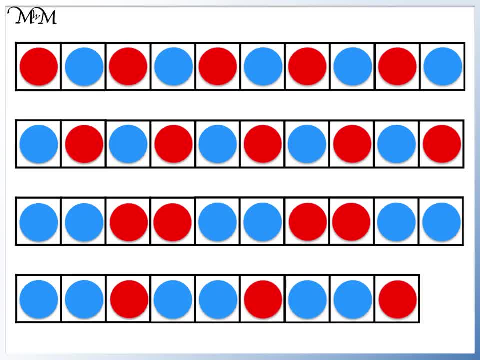 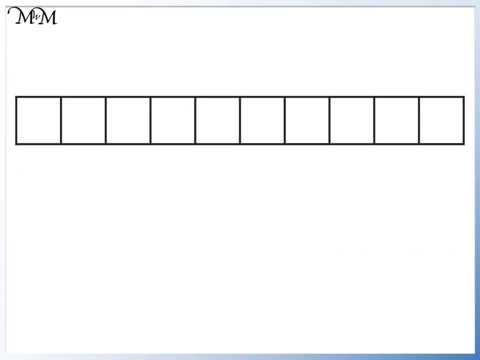 We would now add another blue, blue, red, But we only have space for the first colour, which is blue. This pattern will go: green triangle, green triangle, blue cross. We will make our full sequence by repeating these three symbols. We have green triangle, green triangle, blue cross. 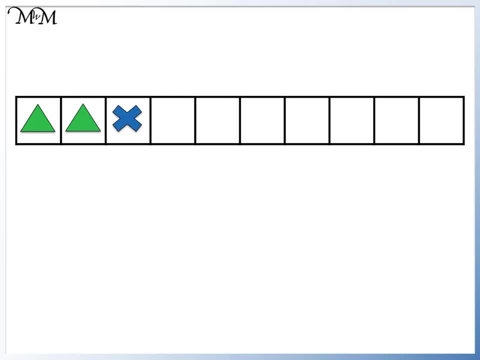 We will put these three down. after each blue cross, Green triangle, green triangle, blue cross, Then green triangle, green triangle, blue cross. We have one space left. The pattern goes: triangle, triangle cross, triangle, triangle cross, triangle, triangle, cross. 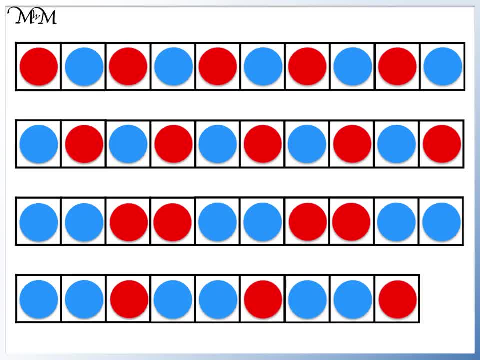 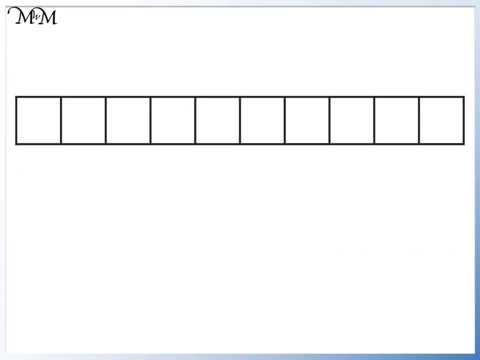 We would now add another blue, blue, red, But we only have space for the first colour, which is blue. This pattern will go: green triangle, green triangle, blue cross. We will make our full sequence by repeating these three symbols. We have green triangle, green triangle, blue cross. 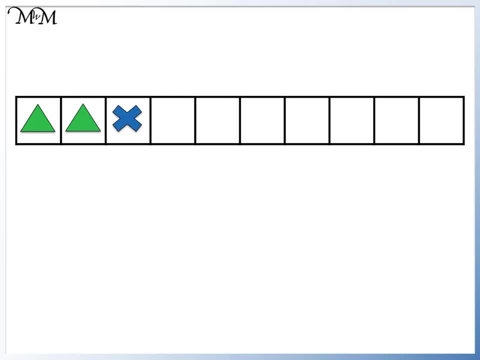 We will put these three down. after each blue cross, Green triangle, green triangle, blue cross, Then green triangle, green triangle, blue cross. We have one space left. The pattern goes: triangle, triangle cross, triangle, triangle cross, triangle, triangle, cross. 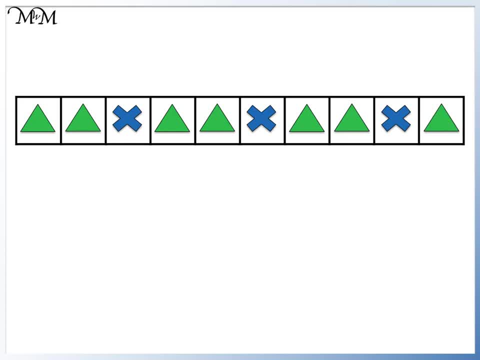 Next is the first symbol in our pattern: green triangle. What is the next symbol in this pattern? We have right, left, left, right, left, left, right, left, left. At the end of the sequence, we have left, left. 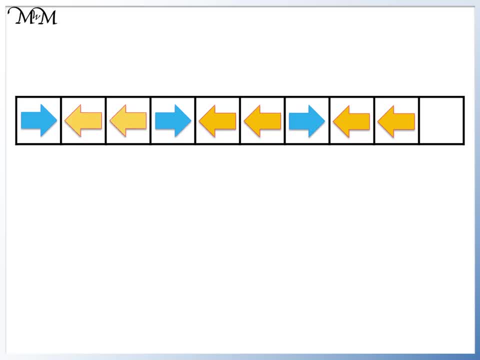 We can see here a left left which is followed by a right. This left left is followed by a right, And so this left left is followed by a right. What is the missing symbol in this sequence? We have two rights. 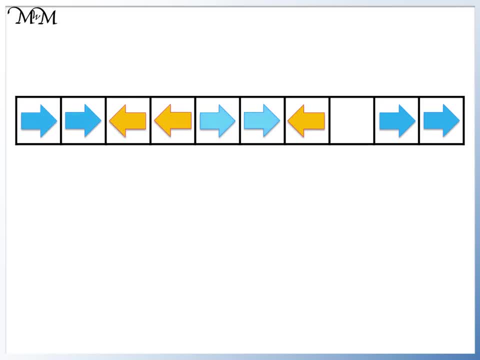 Two lefts, two rights. We have one left and need one more to make two lefts. Now we have our complete pattern: Two rights, two lefts, two rights, two lefts, two rights. What is missing in this pattern? 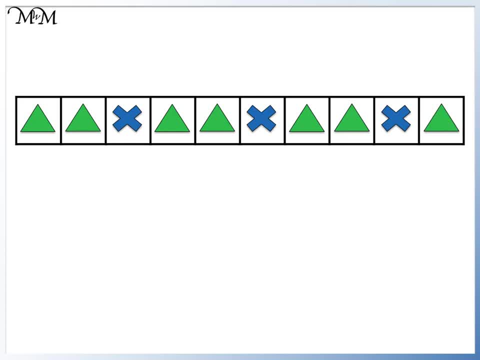 Next is the first symbol in our pattern: green triangle. What is the next symbol in this pattern? We have right, left, left, right, left, left, right, left, left. At the end of the sequence, we have left, left. 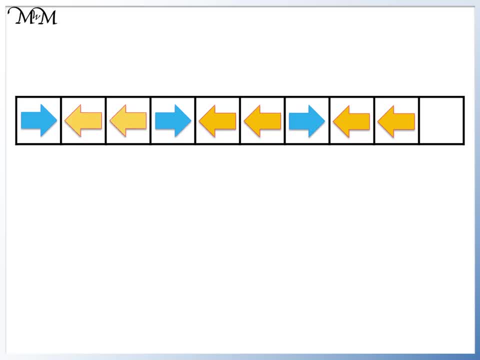 We can see here a left left which is followed by a right. This left left is followed by a right, And so this left left is followed by a right. What is the missing symbol in this sequence? We have two rights. 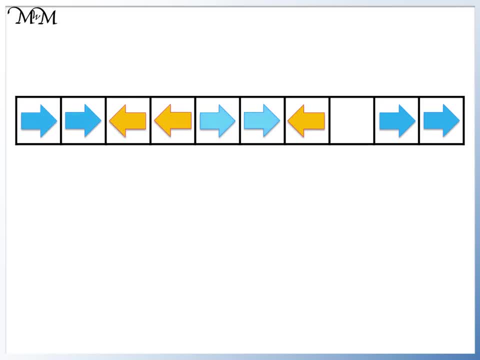 Two lefts, two rights. We have one left and need one more to make two lefts. Now we have our complete pattern: Two rights, two lefts, two rights, two lefts, two rights. What is missing in this pattern? 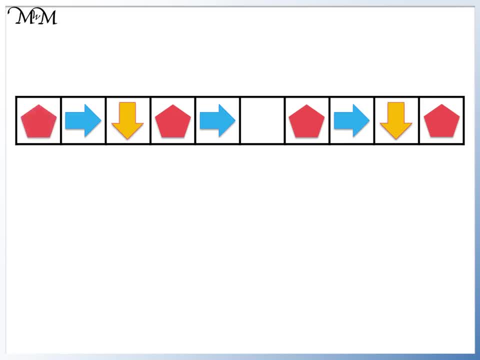 We can see we have red pentagon right down. We get back to red pentagon Further on. we also have red pentagon right then down. So here we have red pentagon right then down. What is missing in this sequence? 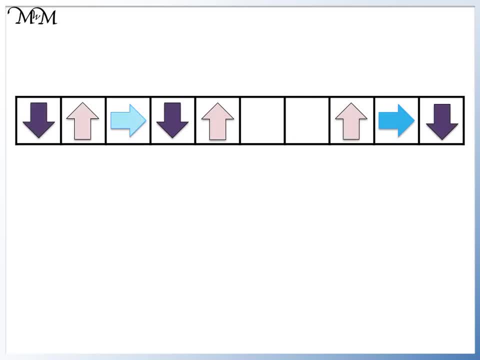 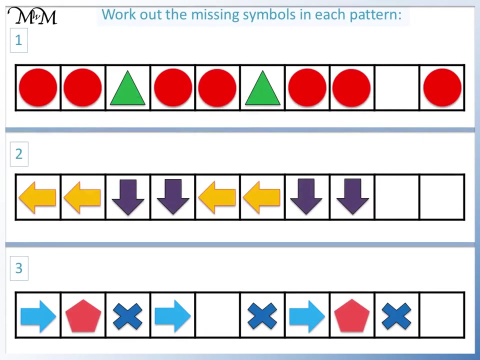 We have down up right, then down up. Later we have up right down. We repeat: down up right. So we have down up right. After right we start again at down. Here are some questions for you to try. 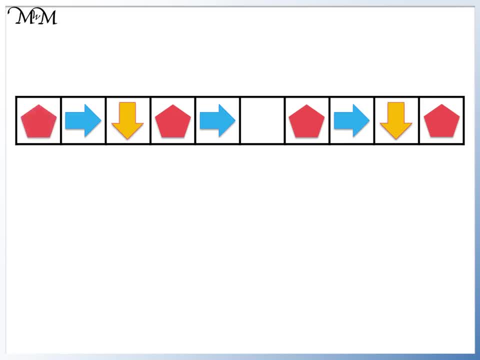 We can see we have red pentagon right down. We get back to red pentagon Further on. we also have red pentagon right then down. So here we have red pentagon right then down. What is missing in this sequence? 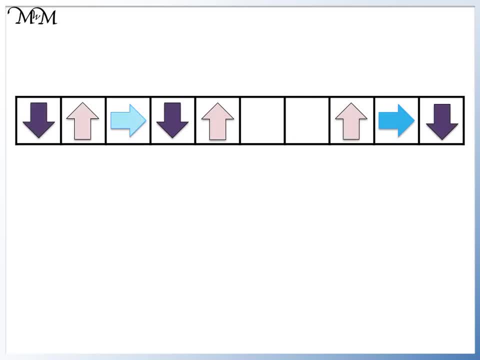 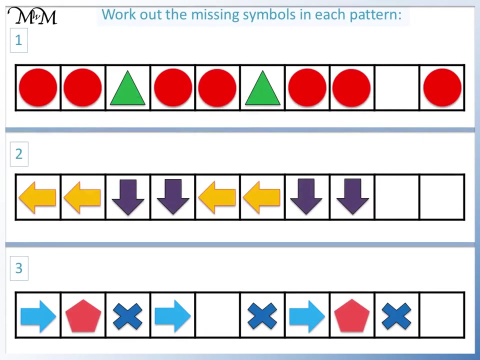 We have down up right, then down up. Later we have up right down. We repeat: down up right. So we have down up right. After right we start again at down. Here are some questions for you to try. 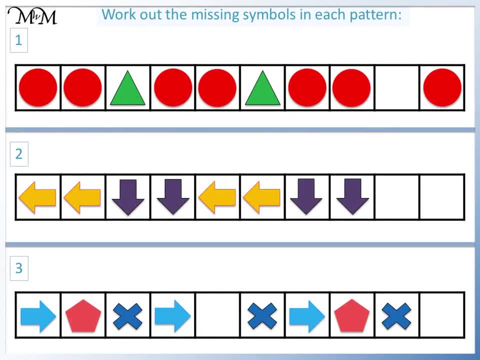 Work out the missing symbols in each pattern. Pause the video and have a go. Question one: We have circle, circle, triangle, Circle, circle triangle. After two circles, we have a triangle. Question two: We repeat: left, left, down down. 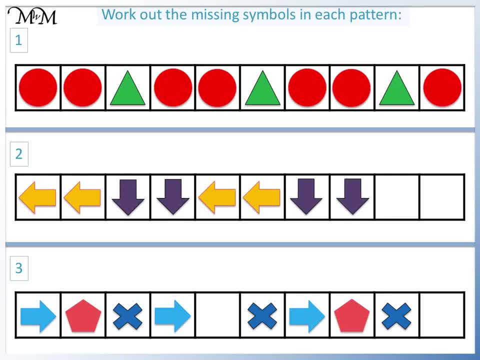 Left, left, down down. Next we have left, left. Question three: We repeat the three symbols: right, pentagon cross. After right, we have a pentagon Here, we have right pentagon cross And we are back to the start with another right. 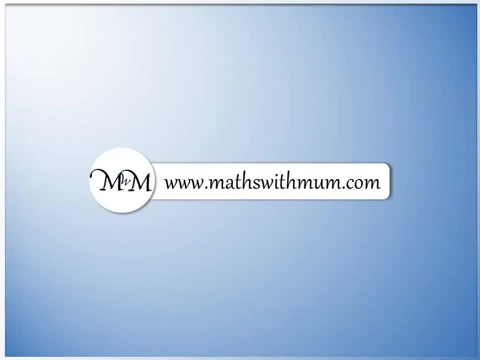 Thank you for watching For further practice. more questions are available on our website.